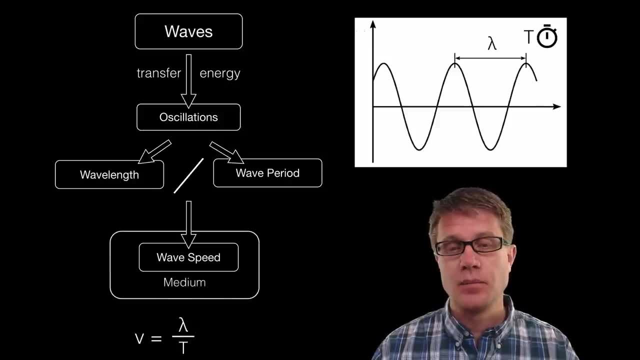 than it does in air. So the medium determines that. But there is an established relationship between the velocity of the wave and then the lambda divided by time, Or the lambda divided by the period. Now, lots of times, since the frequency is the reciprocal of the period. 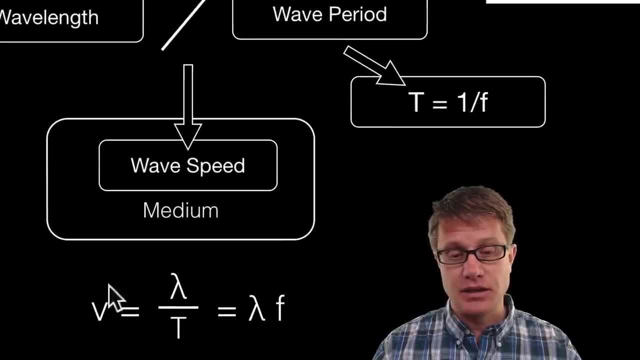 of time, and so, instead of being written like that, it will be written like this. It will be written like this: V equals lambda f, In other words, the velocity or the speed of the wave is the lambda, or the wavelength times the frequency. And so let's take a look at. 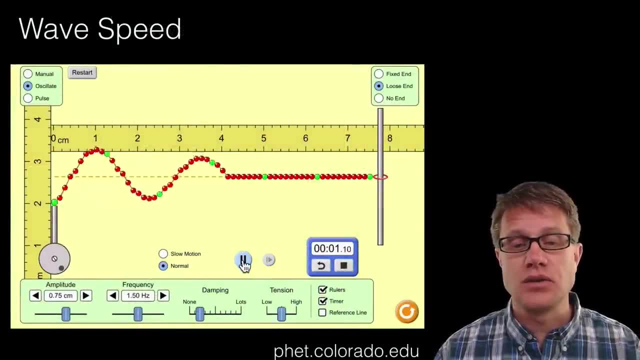 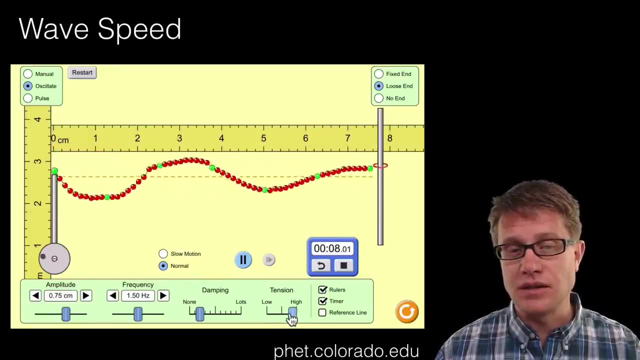 that wave speed for a second, And so we will just do this qualitatively. So what I am going to do is start some waves in this simulation And then I am going to play around with the tension And watch what happens as I make it less tense and then more tense. I could 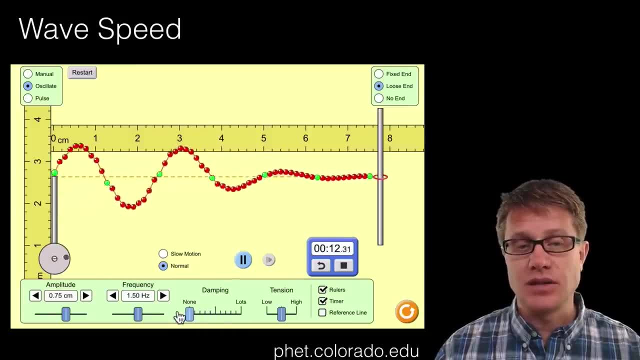 also affect how much of it is being dampened by the medium itself. And so you can see that I can play around with the medium itself And I can vary the frequency of the wave. So I am going to play around with the wave And then I am going to play around with the medium itself, And then I am going to play around with the wave itself, And then I am going to get the velocity, which invisible by the magnitude of the radius of the wave, And then I can look at what this is going to look like, something like I am running this: 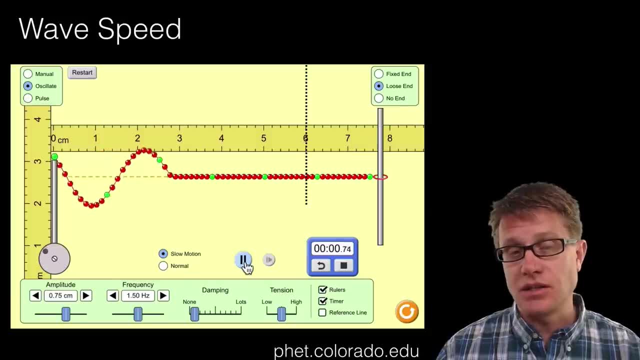 whole simulation where one wave is moving But the density is going to be the speed of the waves. So let's just look at one for a second. So we are going to keep that tension the same, But we are sending one wave down And we will stop it right when it gets to. 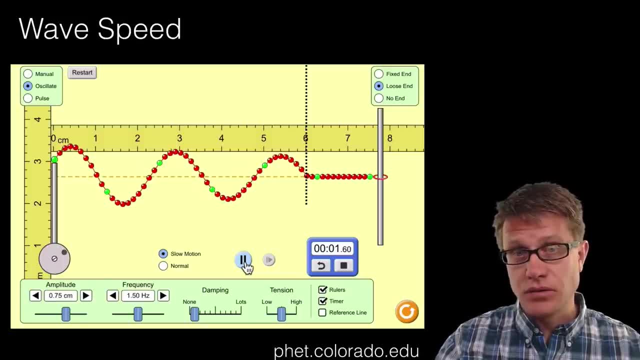 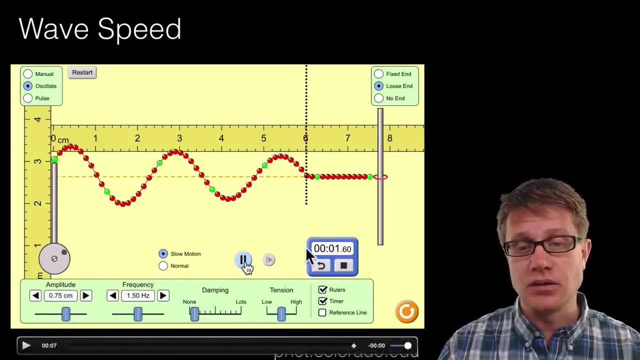 6 centimeters, And so now we have watched the wave move, So we are going to try to calculate wave speed in a couple of different ways. So it has moved a set distance from here to here, And again I had the clock running, So it took 1.6 seconds for it to make it there. 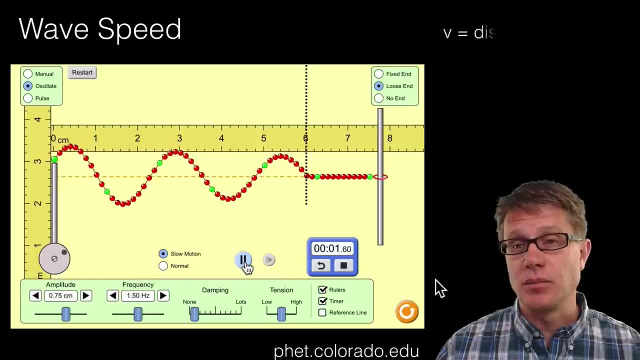 And so if I want to figure out its wave speed, some way to do it was to measure distance divided by time. So what is the distance? And this can take either two or more seconds distance. In this case we moved 0.60 meters per 1.6 seconds. You can see I converted that. 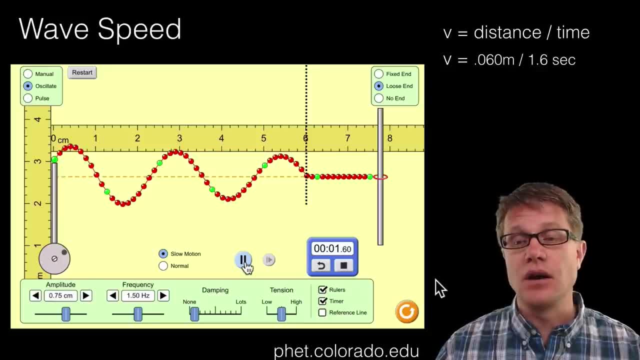 to meters, And so what is going to be the wave speed? just watching the wave go, It is going to be around 0.038 meters per second. Now we also know that you could calculate it in a different way, And so velocity equals lambda times, frequency, And so we could calculate. 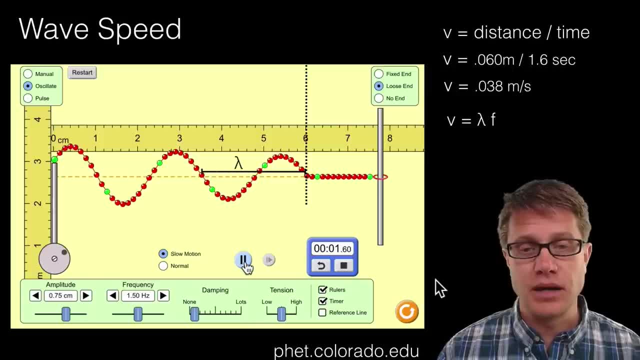 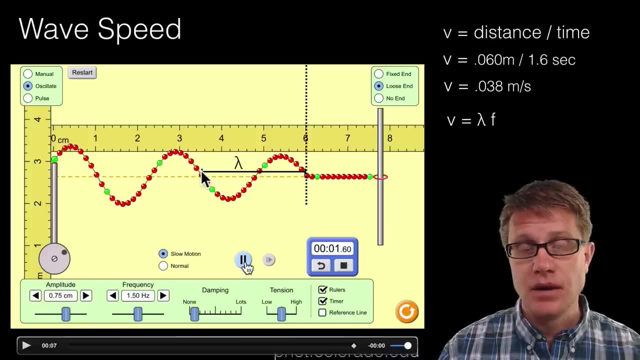 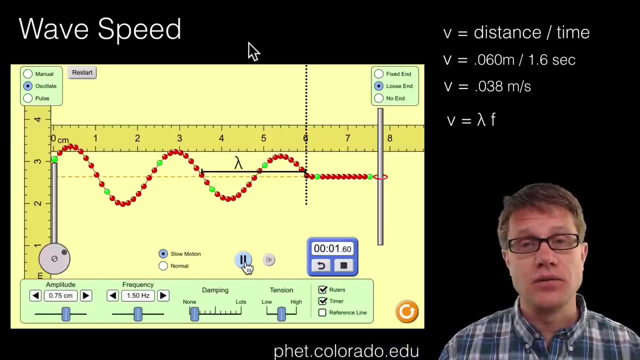 lambda. Lambda is going to be the wavelength, So let's figure out what the wavelength is. So from here to here, it is 1 to like 2.5 centimeters. And also, on this simulation, it is telling us what the frequency is. And so if I know the frequency and I know the wavelength, I know. 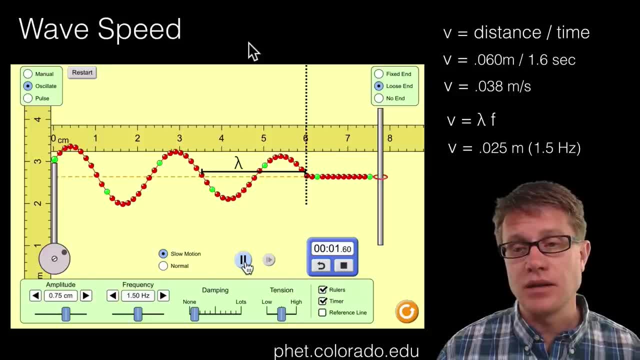 the velocity, And let's make sure that that matches. So my wavelength is 0.025 meters, My frequency is 1.5 hertz, And so it is going to be 0.038 meters per second. So same thing. 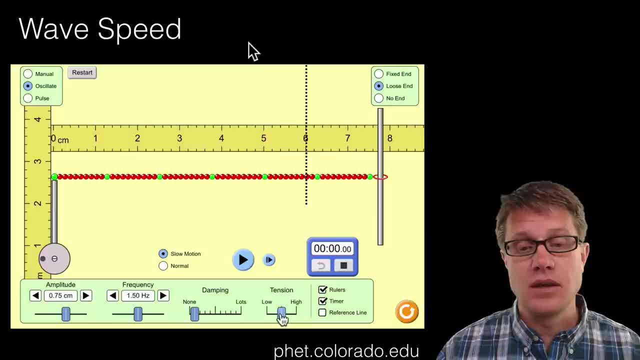 We could then try to change the makeup of the material or the matter through which the wave is moving. So let's start it now. So we have increased tension, So it went faster. You can see the time is less, So it is 0.96 seconds, So we could calculate. 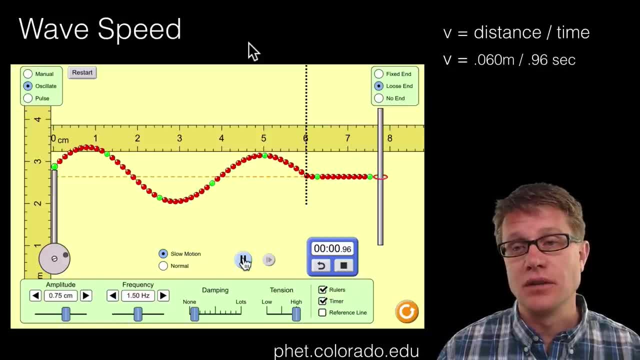 the distance we moved Again, that is 0.060 meters per 0.96 seconds. So that is one way, So we could get a velocity that is much faster than it was before. So as we increase tension, we have increased the speed. But we could also use: v equals lambda f, And so what is? 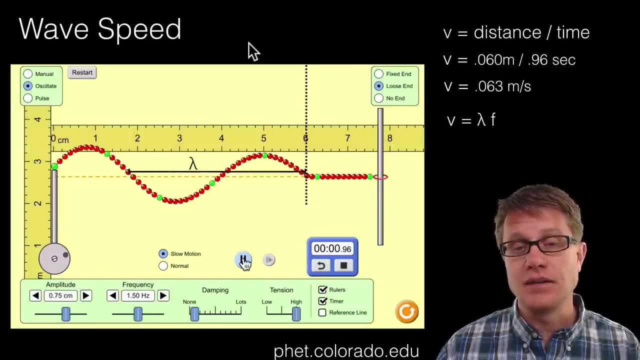 our lambda, what is our wavelength, What is our velocity, And so we can calculate the velocity. It is going to be that distance, And what is our frequency? 1.5. And so we could say it is going to be the same value. And so those are two ways we could calculate. 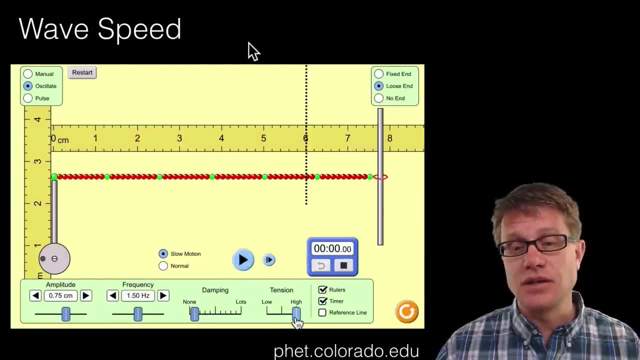 the speed of the wave. Now what happens if we totally decrease the tension? There is no tension inside there. Oh, you can see that it is going really, really slow, And so I am not going to keep going on this one. It would take forever. And so, as we increase, 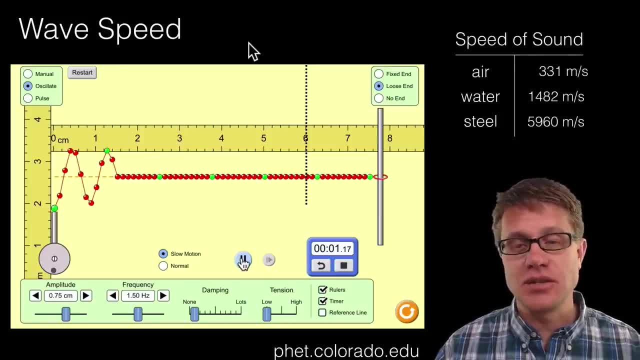 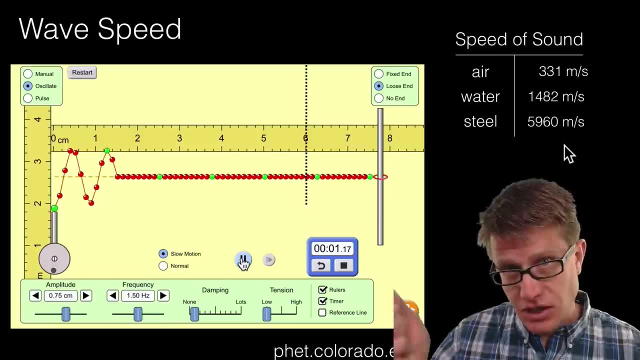 the tension inside the material. you can see we are increasing the speed. So here is some speed of sound. So this is an air 331 meters per second. This is an air 331 meters per second. In water it is much faster. And in steel, if you were to just hit steel and then 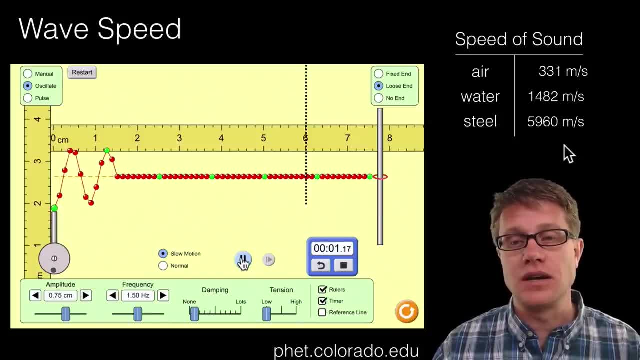 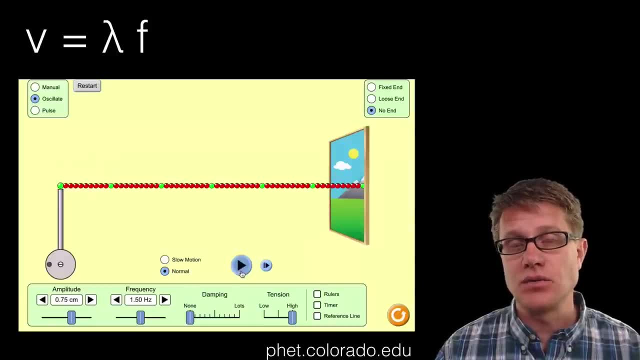 listen to it. really far down it is going to go way faster than it would inside the air itself. Now let's say we keep the medium the same. Let's say we keep the tension and everything the same. What is going to be the relationship between the wavelength and the 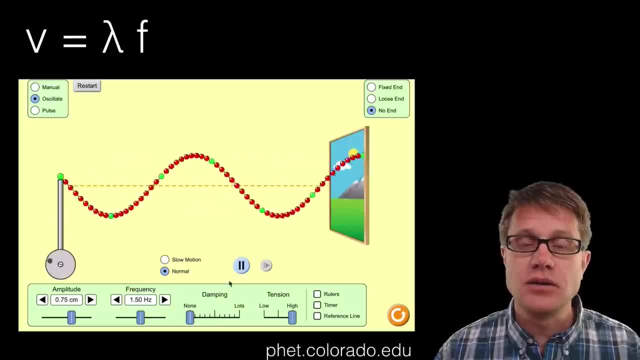 frequency of the wave. And so let's just start it going, And what I am going to do is vary the frequency. And so as I increase frequency, what happens to the wavelength? You can see it decreases As I now decrease frequency. what is going to happen? Well, I am going. 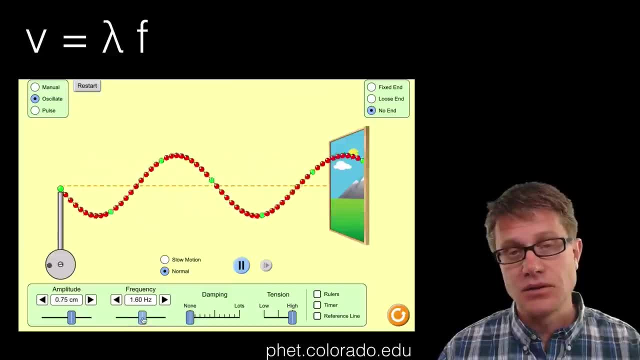 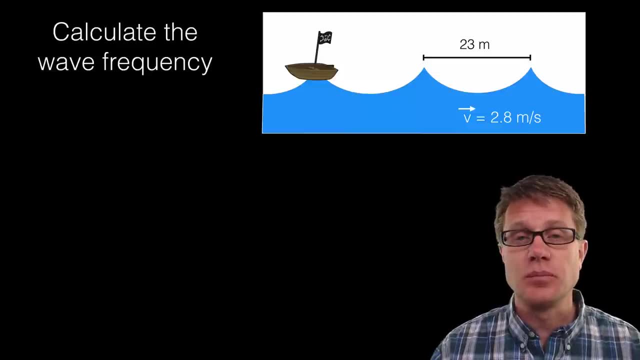 to increase the wavelength. Now you can see the wavelength is increasing. So again, the medium determines the speed of the wave, but then there is this relationship between the wavelength and the frequency. Lots of times you will be given problems like this. So for